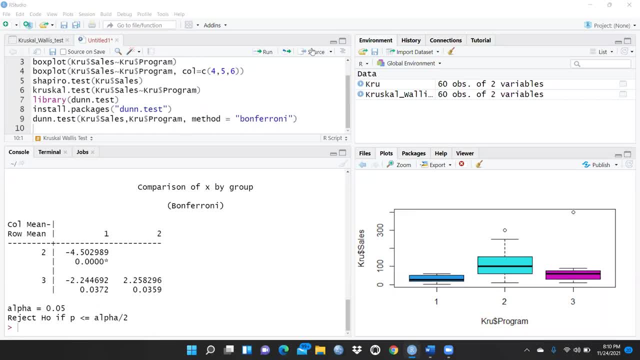 Hi everyone, let's begin our new test, Kruskal-Wallis test, and it is a non-parametric test. So how we have to perform this test? and basically it is the replacement of one-way ANOVA When we have one sample. here is Kruskal-Wallis test. allows possible differences between: 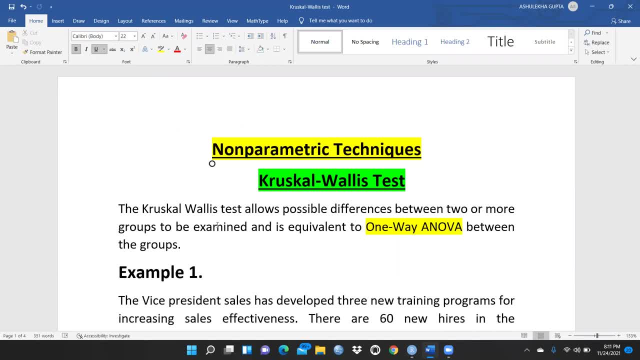 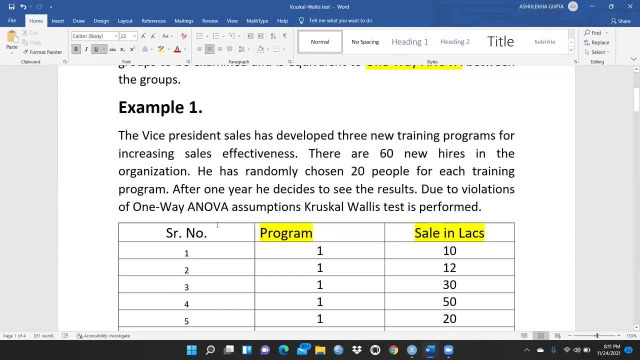 two or more groups to be examined and it is equivalent to one-way ANOVA between the groups. So I have taken one example. The vice president, sales, has developed three new training programs for increasing sales effectiveness. There are 60 new hires in the organization. 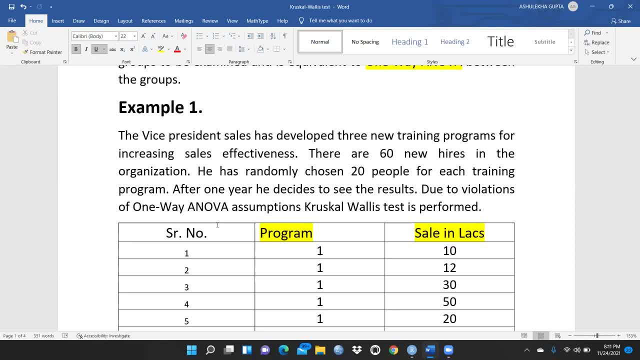 He has randomly chosen 20 people for each training program. After one year he decides to see the results. Due to violations of one-way ANOVA assumptions, Kruskal-Wallis test is performed. So, first of all, we will understand why there is one-way ANOVA assumptions violations. Why? Because 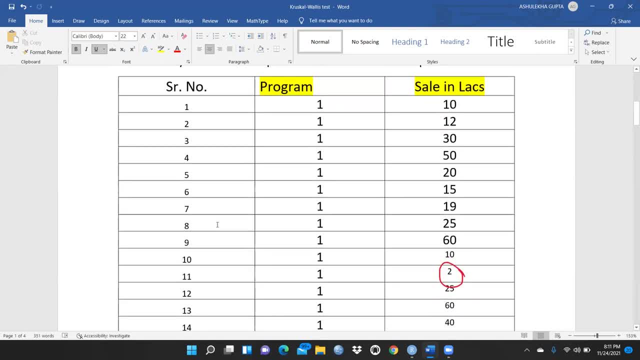 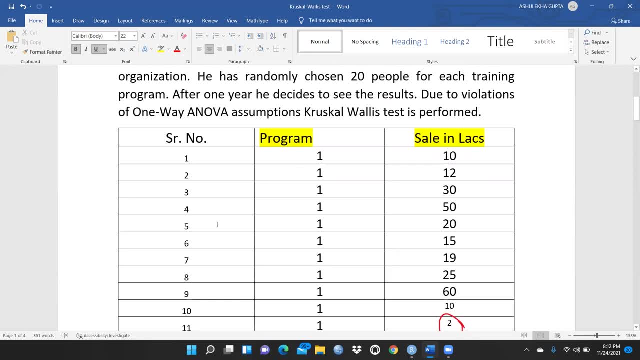 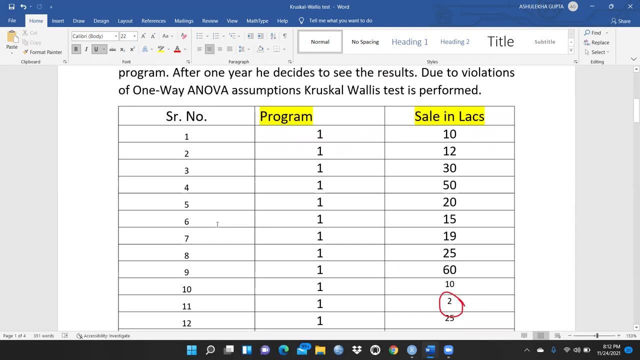 this data is not normally distributed And here is you can see program that is categorical data and sales in LEX. that is our continuous data, that is ratio scale, that we have got this data, So we have a metric scale, but program is: you can see one. then second training program: 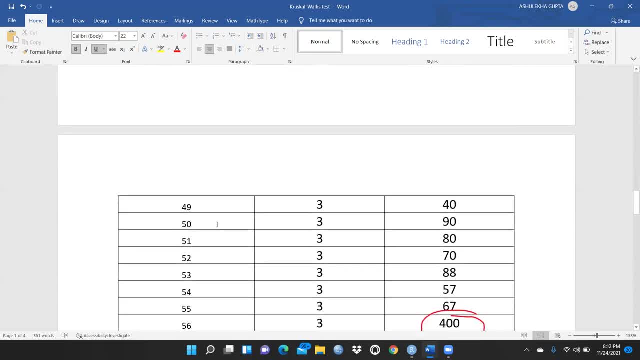 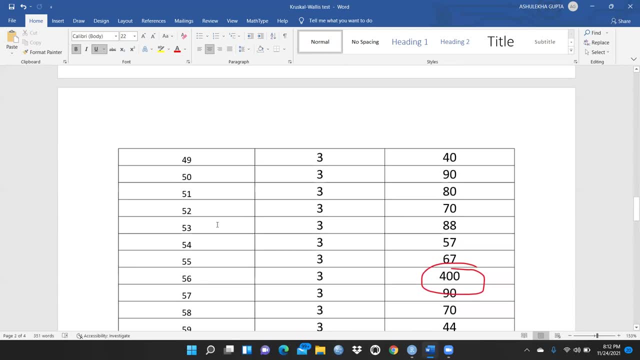 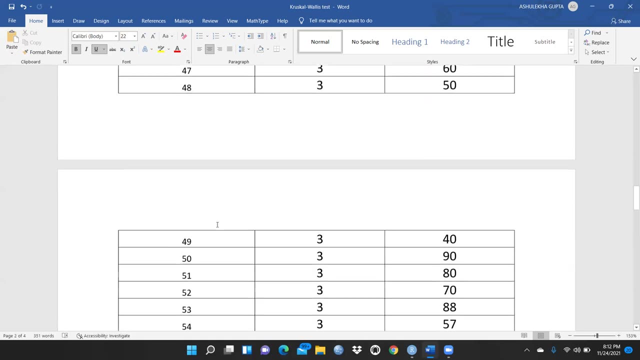 is two and third kind of training program is three. So total number of the new employees are 60.. So we are- and this is the independent kind of sample, because there is no relationship of first 20 employees with second category of employees than the third category employees- 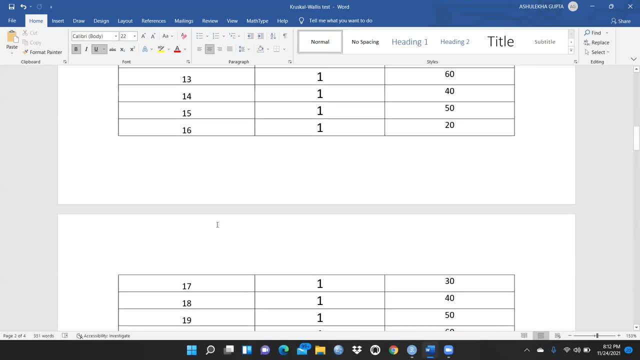 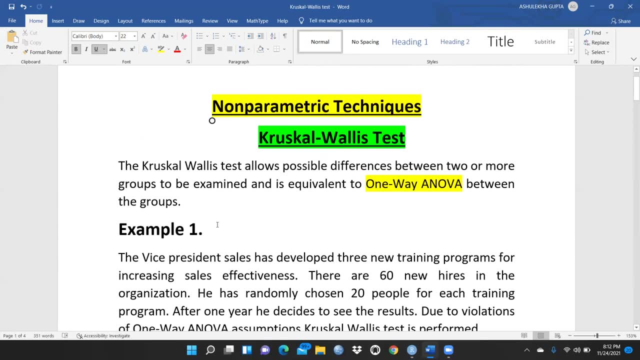 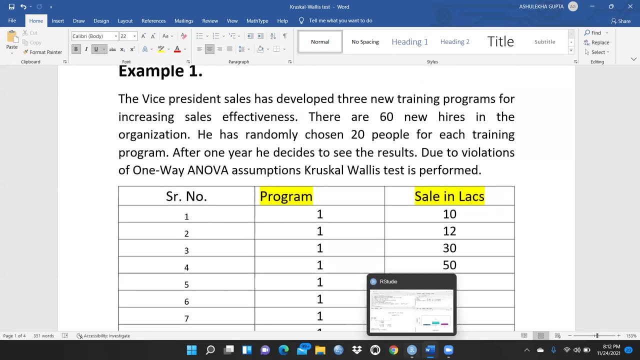 These are the independent samples. So what we have to do this is non-parametric. So that is why we are not normally distributed And that is why we are going to apply this non-parametric technique. So let's begin this. in our studio, I have already done something. 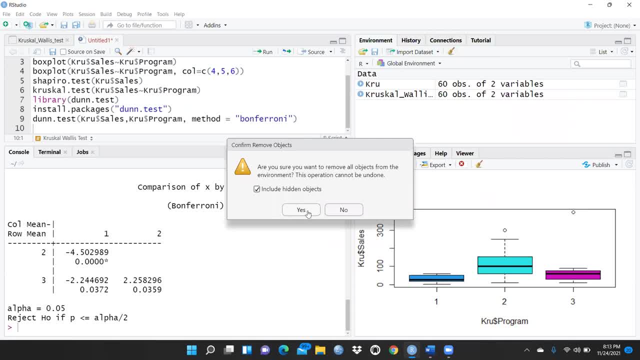 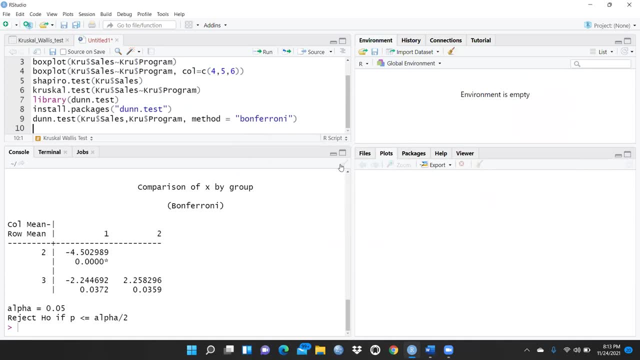 So what we have to do: let me clean all these windows, all these graphs also, And let me clear this. And here is all this. So I'm just I'm just clearing this new file also. So, first of all, what we have to do: first of all, I'm going to import dataset and my 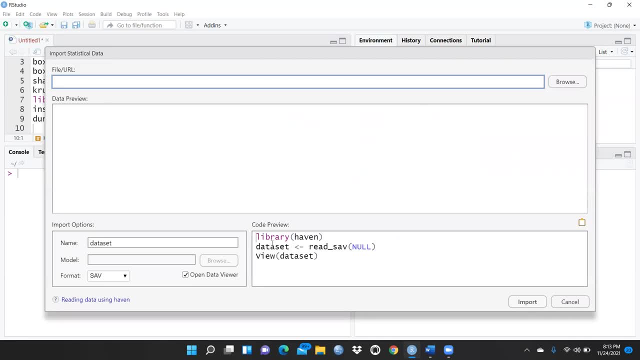 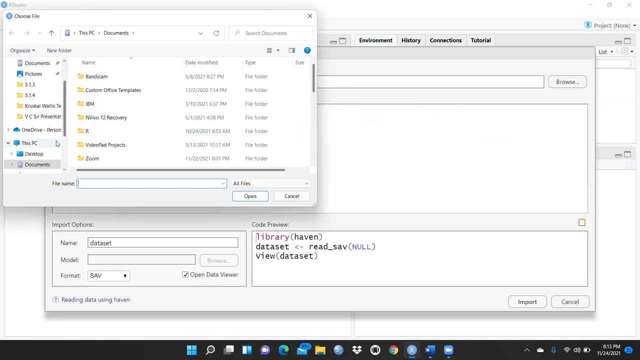 file is SPSS kind of file. So I had already explained you library heaven is required And what we have to do. where I put it, my file. let me check. Okay, Fine, Crisco Wallace test in this folder. I had put it this file. 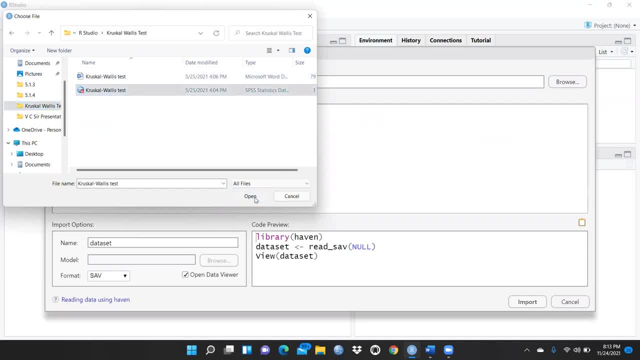 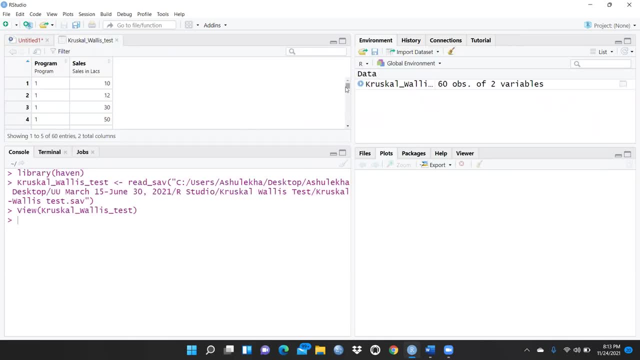 And this is my SPSS file. So let me open this file and let me import this file. Now you can see same data that I had reflected on the word document. that is reflected here. All 60 entries are here. 60 employees data but 2020: each group. 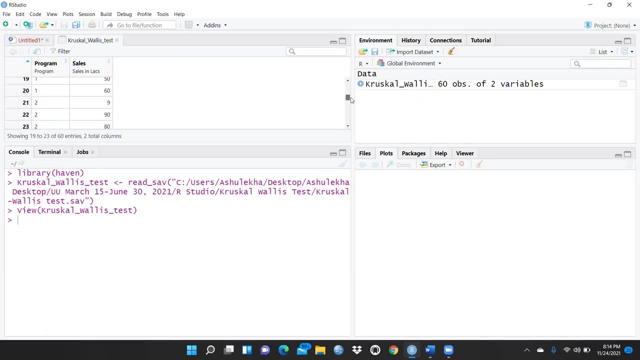 I mean first 20 entries. those have got training number one. two, I had given training number two And Number three, I had assigned training number three. So you can see, and this is the sales right, When they have got, when we had provided this kind of training, what is the sales? 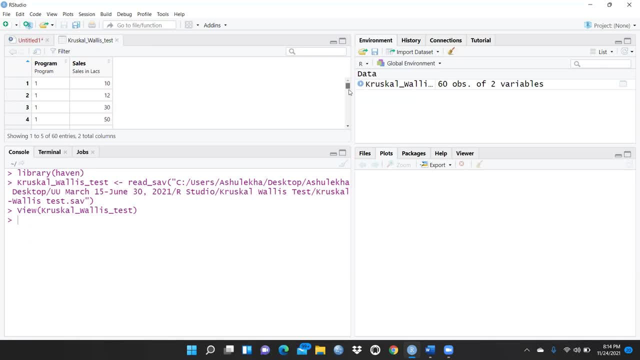 What is the performance right? Sales in Lex And when we had provide second kind of training. so what kind of sales we are getting? So what we have to do: first of all, I had already imported this file. What we have to do. 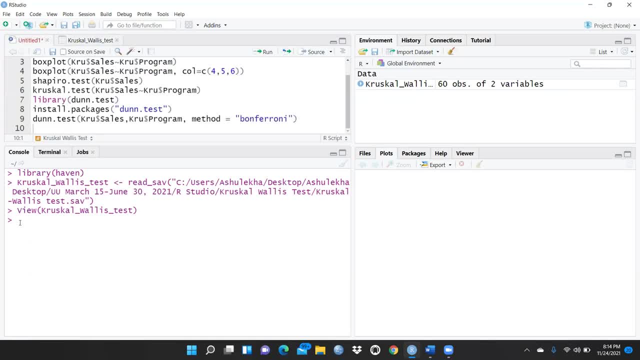 Let me create one new variable over here. Let me write K R U right And in this particular variable, let me put this file: And what is this complete file name is Kruskal. yes, This is the my file name: Kruskal Wallace test, and I have to press enter. 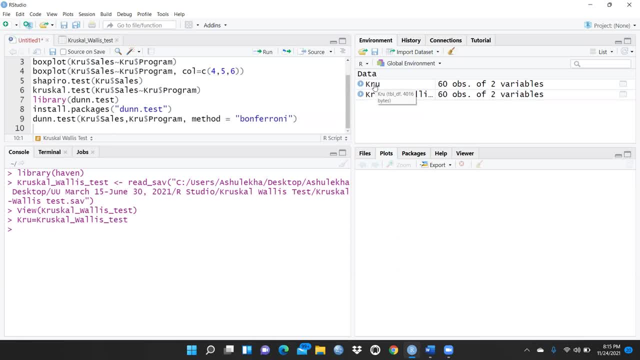 Now you can see this new variable is put it here. So now we have to use this, the small name of this file, rather than this is the bigger name. Okay, So what we have to do, we can. first of all, what we have to do. let me first check whether 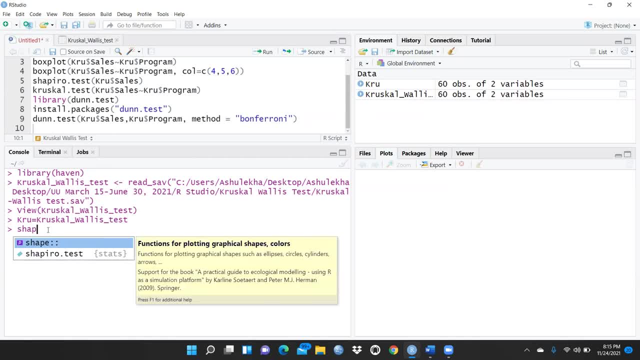 this data is normally distributed or not. So what I have to do is Shapiro test and Shapiro test off. I have to apply. that would be on the this crew now new file name, new variable name is crew and I have to write dollar sign. 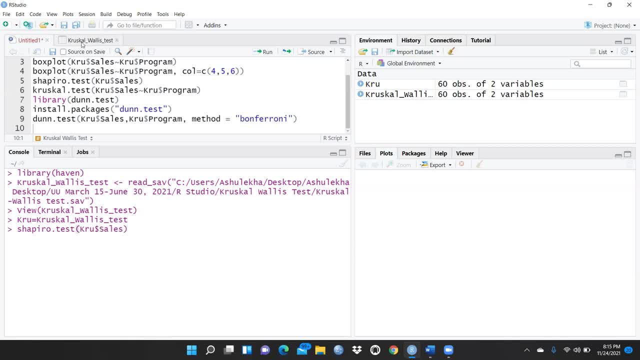 And this is the continuous variable. right, Sales is only continuous variable. You can see here That is only in numbers. This one is the categorical variable. So what we have to do, let me enter this and you can see: Shapiro week normality test and. 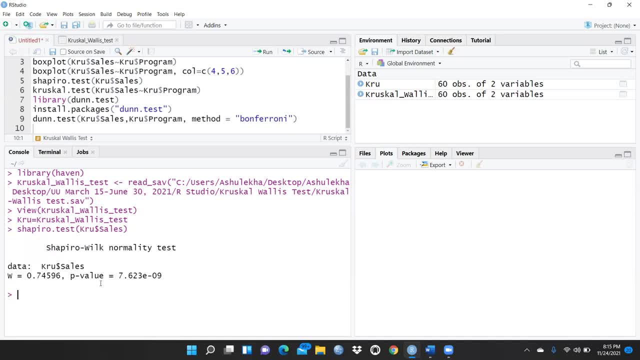 this is very, very less than 0.05.. So we can see our data is not normally distributed right. And here is we can apply this test also, homogeneity test also. And again we have to write K R U. 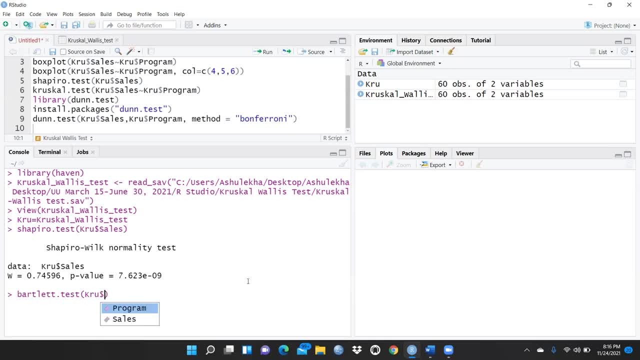 This is my file name and I have to write dollar sign And again I have to write sales and I have to press enter. now, Okay, Fine, There's the some mistake. Okay, Okay, Okay, Okay, Let me, I have to write this. 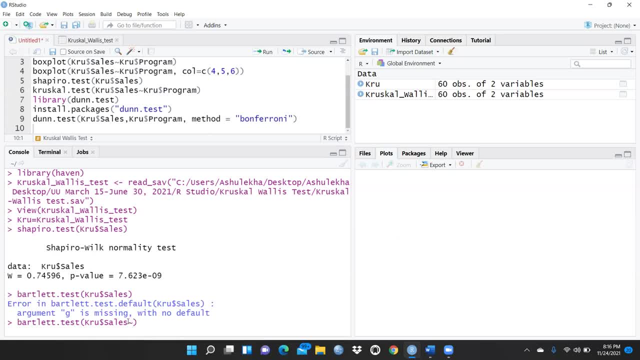 Then I have to: Yeah, And I will write again the same file name: K R U. and here is: we have to write dollar sign, and then I have to write program, and then we have to check homogeneity of this test. Right. 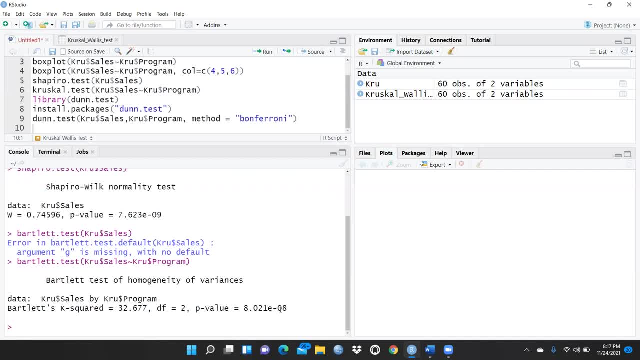 Then again you can see here, the P value is less, less than E- to the power zero eight, That is less than 0.05.. Then that means this data is not homogeneous. So both these conditions are fulfilled. That is why we had applied Kruskal-Wallis test rather than one-way ANOVA on our data. 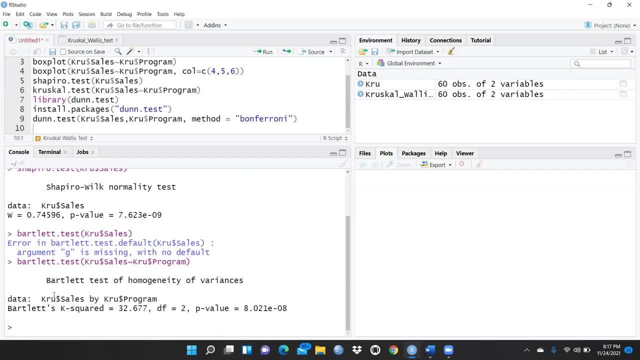 sample Now what we have to do through boxplot test also, we can apply this right. So we have to write boxplot and what we have to do. let me take this K R? U. This one is the my file name and I have to write dollar sign. 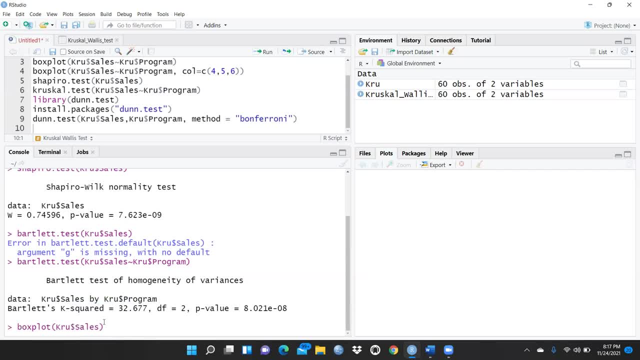 Then I will write sales, right, sales and a boxplot. I want both these variables, both these, both these parameters. So what I have to do, again I have to write this one is the file name, And again I have to press dollar sign, and then I have to take program right. 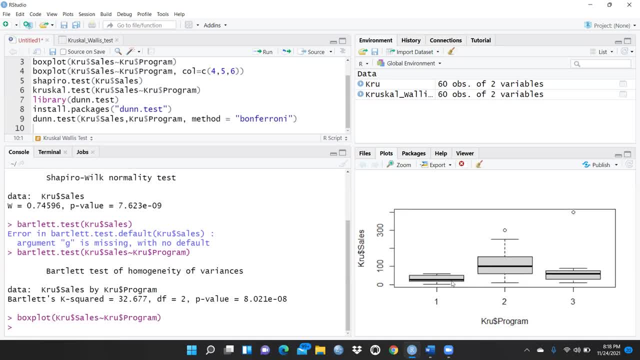 And simply I have to enter this So you can see three box plots are here and itself they are defining. I mean these, this. this data is not similar And there's the lot of variation in these three training programs: one, two and three. 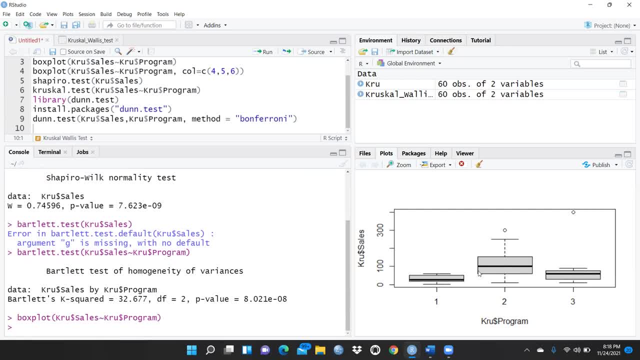 You can see here the mean value of this second one, And when we are giving only one training, first training, and when we are giving third training, training number three. So what we have to do, let me give this particular box plot right. 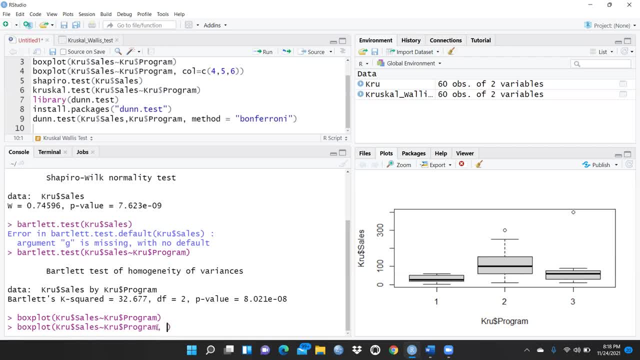 Let me assign one color also So there would be easily We can Distinguish. So let me write C O L and what we have to do, C O L. and let me write C and what three colors we want to give. let's say I am giving five, six, seven. 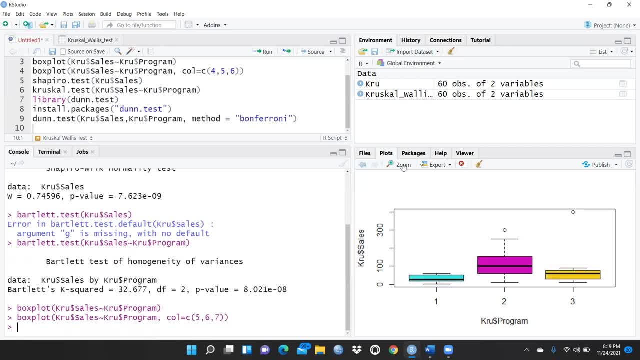 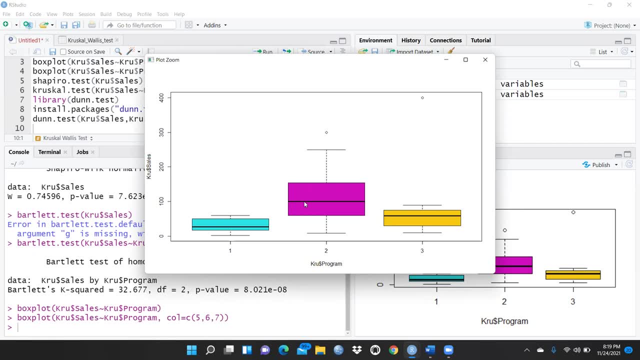 These are the color codes I want to give So you can see here when we can zoom this. these three colors are here and you can see lot of difference because mean value. You can see middle one is on the higher side and that is on the very lower side. 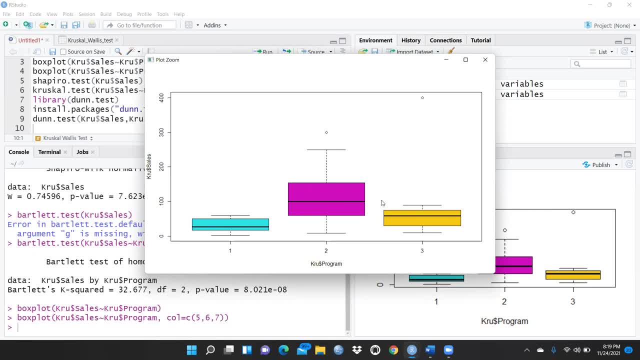 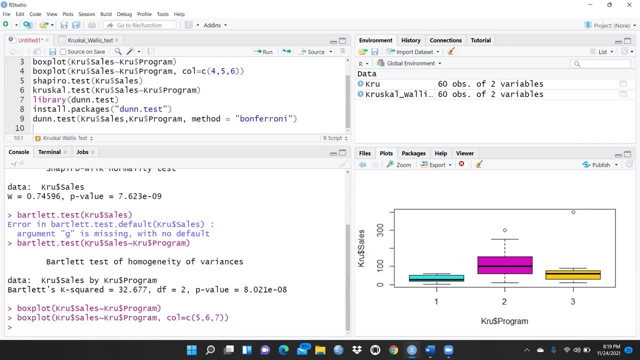 But the third training that shows is on the little bit and all this data is not, uh, normally distributed. So now, all the tests we we have done, now what we have to do, we will write this crystal before writing this crystal. 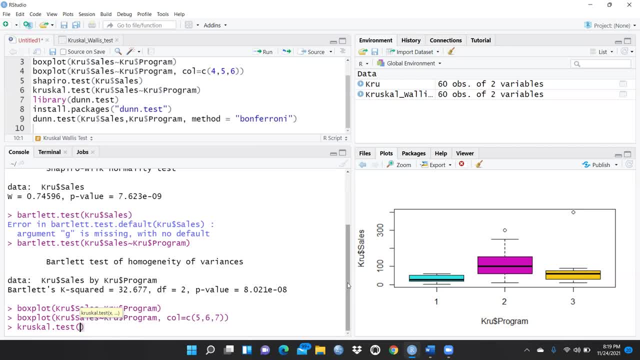 Okay, Fine, Crystal test, Right. And what we have to do? Crystal test. Now. We will write K R U again the same file name, and I have to press dollar sign. Then I would- uh, I will select this: seeds. 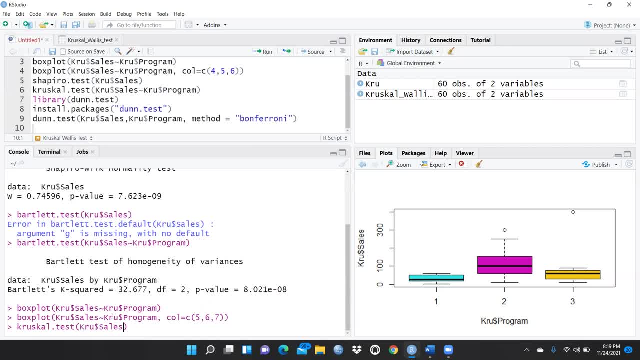 And after that what we have to do here is we will again enter the still sign And after that again we will write crew K R? U and again dollar sign, And then I will write two grams and I will press enter. 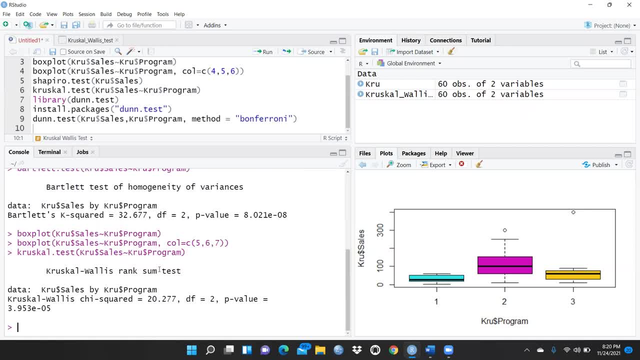 So now you can see. So now you can see Kruskal-Wallis rank, some tests and you can see results of the chi-square is 20.277, degree of freedom two and P value is 3.9 to the power E to the power zero five. 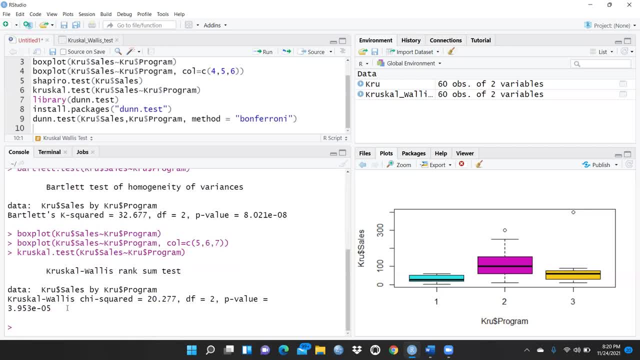 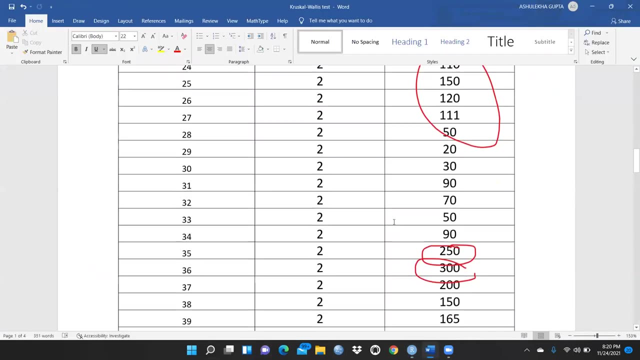 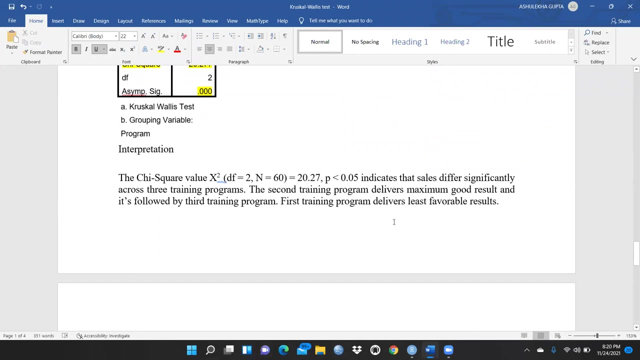 That means it's very, very less than 0.05.. So we can see right, Because when the a P value, P value is three point nine five three E. So here is we can see our hypothesis in the award document. i will show you. uh, yes, we can write this interpretation like: 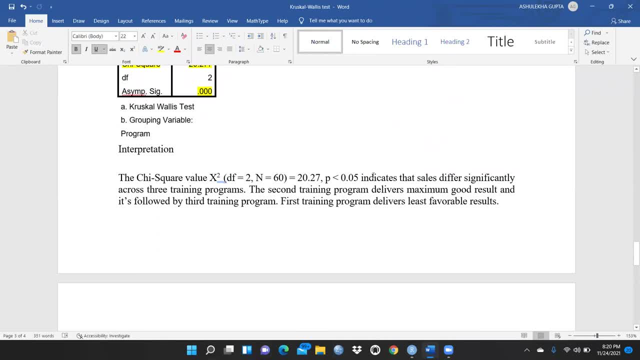 this, the chi-square value degree of freedom 2 and number is 60 and 20.27 and p value is less than 0.05, indicates that sales differ significantly across three trading programs. otherwise, null hypothesis was that there is no significant difference among all the when after providing. 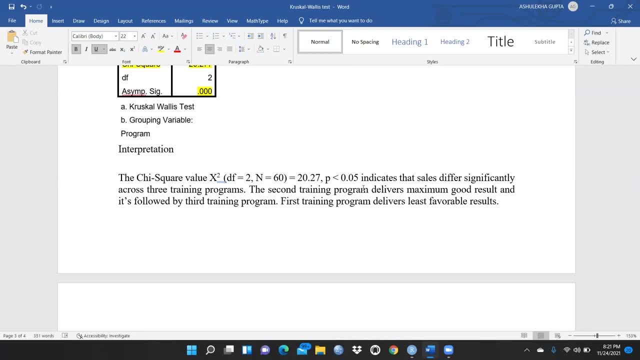 this training program there is no difference in the sales, but here is what we have to do. the second training program delivers maximum good results and it's followed by the third training program. and first training program delivers least favorable results and through our spss also, i have shown you this one is sp, so these are my spss results and when i had 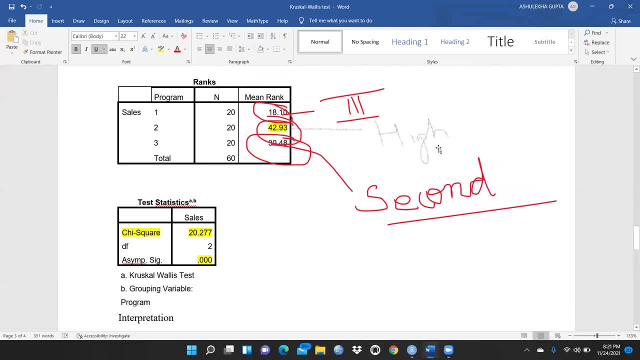 applied sps and definitely i am going to give you link in my description box where i had applied spss. through SPSS I have tested this Kruskal-Wallis and you can see here, let me clean this. I mean, okay, let me clean all these things. second and high right. so now you can see what is happening. 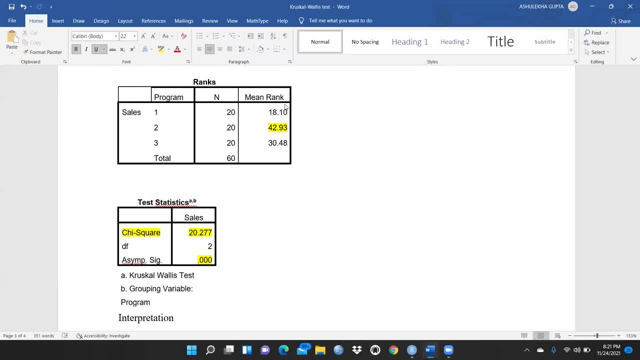 here. this one is the least right. that is very that is on the third place and best results are coming through second training program and the third one is on the second position and the first one when the first training program is giving the very lowest results and that is on the third place. 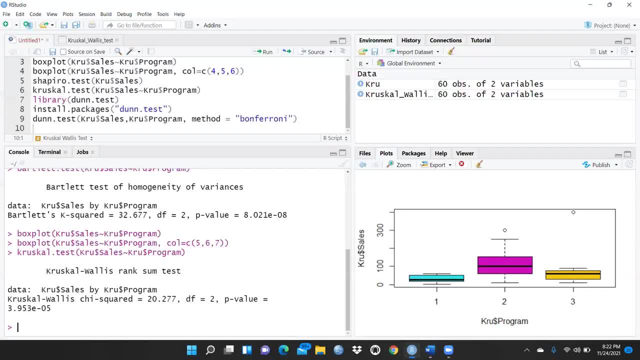 now suppose we want to do in R also. so what we have to do, we will post hoc test, we will apply, because we when we want to distinguish among all three training programs. so what we have to do, let me first install. right, I had already installed, but I have to show how you have to install this package, because we require this. 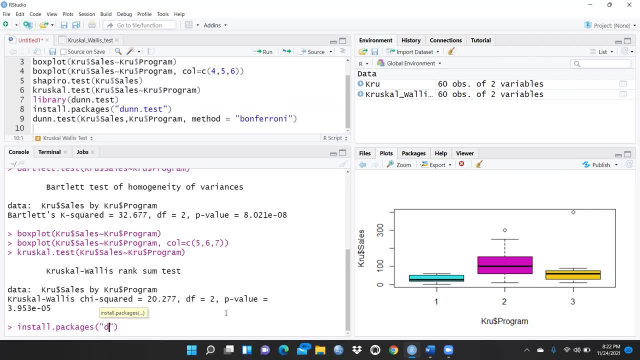 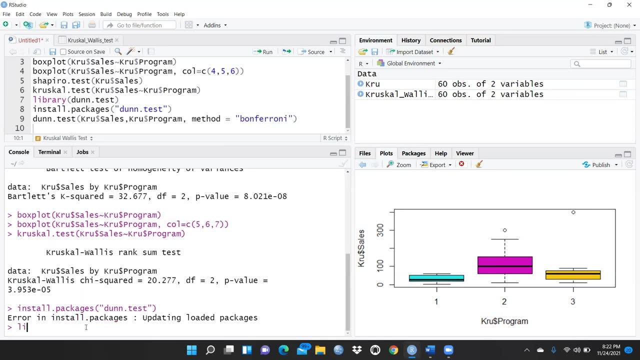 package and simply what we have to do: d u n n done. dot test right. this package we required, so simply we have to write enter. okay, because I had already installed currently, so this message will give, so let me now I have to. first of all, if you want to check, so you have to check through library. 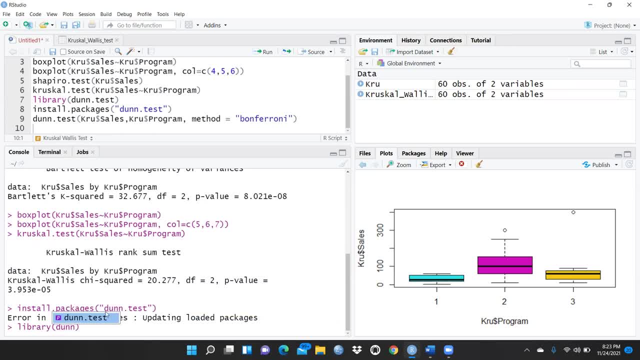 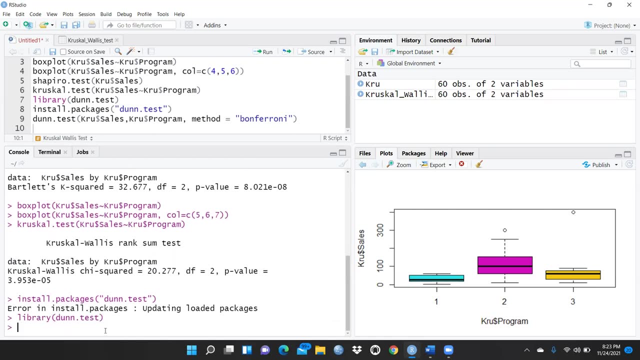 d u n n dot test and if it is available, automatically you can see here. that would reflect. if it is not available, right, you have not installed that library, you have not called, so it will not reflect over here. so, but in my case I had already installed, so that would be reflecting here. so now, 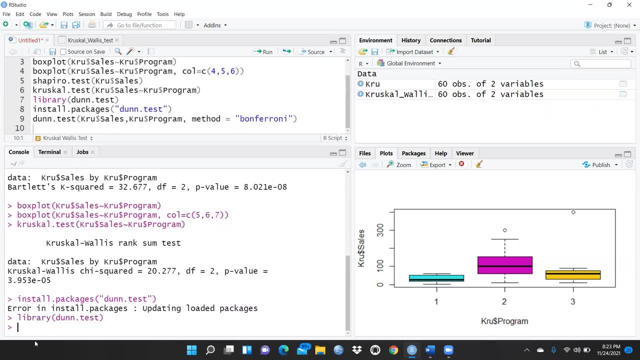 what we have to do for the post hoc test. I have to write done dot test. simply, you will select this right, you will select this and you have to again: right here you, right here you. this is my final name, and I have to write dollars sign and here, as you will write sales comma and 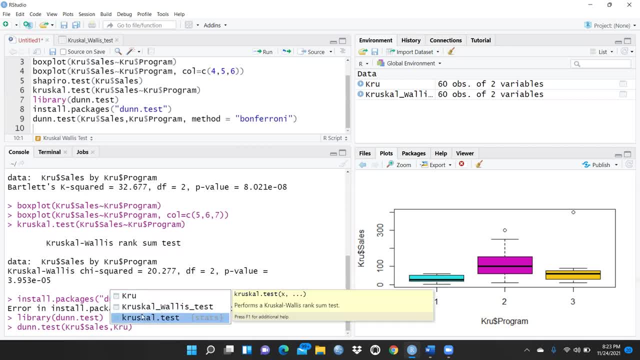 then again same file name you have to write, and again you will write dollar sign, and then here is, you will get the program and once again this filename you should have noted. and then here is 003 and your purchase is ready. so let's paste it back into the data server later and for this set this speed locally once signature was ticked and then here again hit left and then also check our Ground capture again. jednak, can we have all these light up messages now? this 상태 malo. So if you are not so smart, so you just let me say thank you. annoying, because I will contact you for about so many stickский testimonies together. and this is up to date. now, if there is but other people, all right, but any number of business, sí, dans stuffing ny mar. 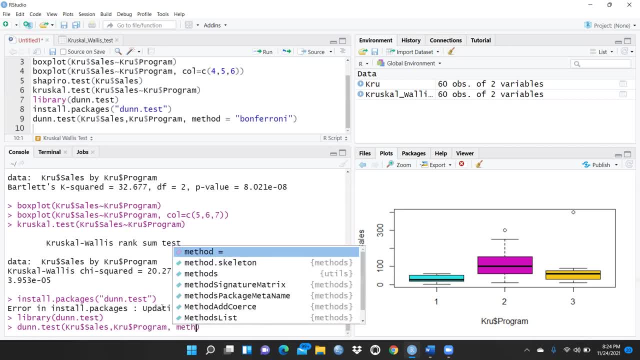 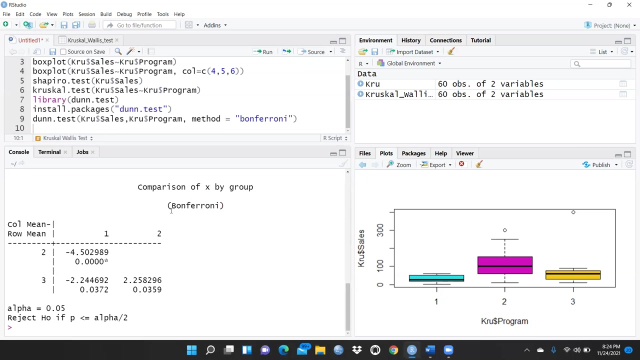 get the program and what method you require to run this postdoc test. simple here is: we have to write here bonferroni test, we require, bonferroni test, we required, and simply now i have to press enter. so now you can see these. comparison of the x by group. right, this is the you can see.